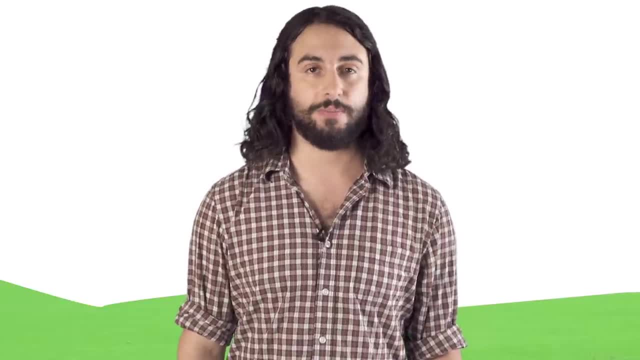 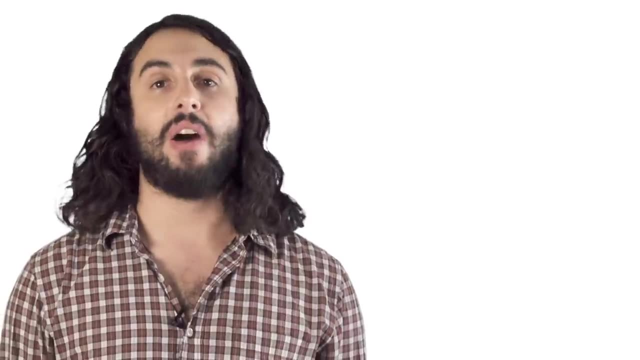 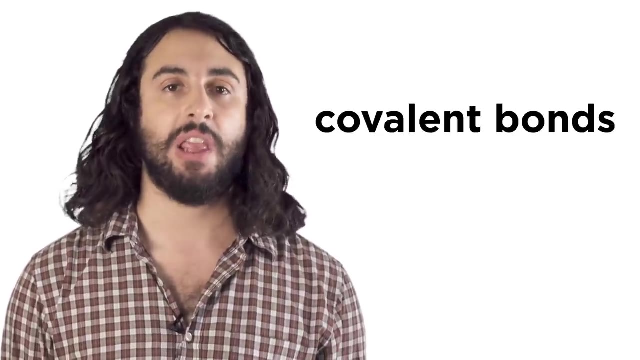 Professor Dave, here let's learn how to draw Lewis dot structures. We've learned about how ions come together to form ionic compounds, but much more interesting is the way atoms form networks of covalent bonds. In order to talk about this, we're 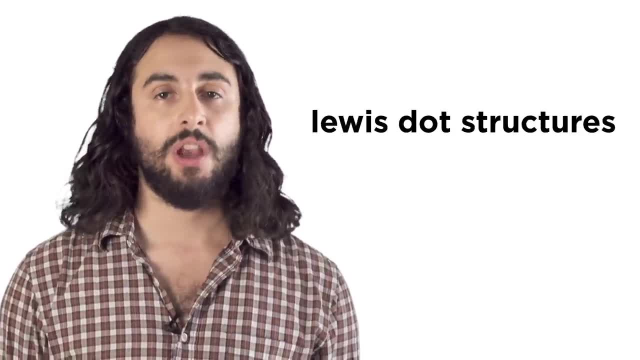 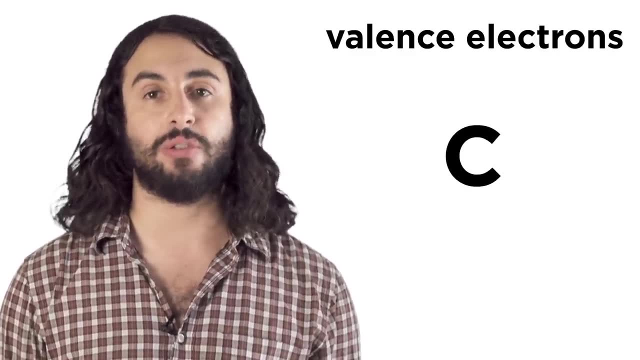 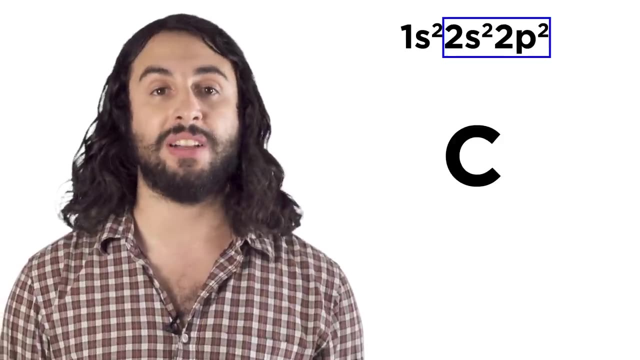 going to have to learn how to draw Lewis dot structures. When we draw these, we will represent an atom by its chemical symbol, here's carbon. we then draw that atom's valence electrons as dots around the atom. carbon is 1s2, 2s2, 2p2, so that's four electrons in the outermost. 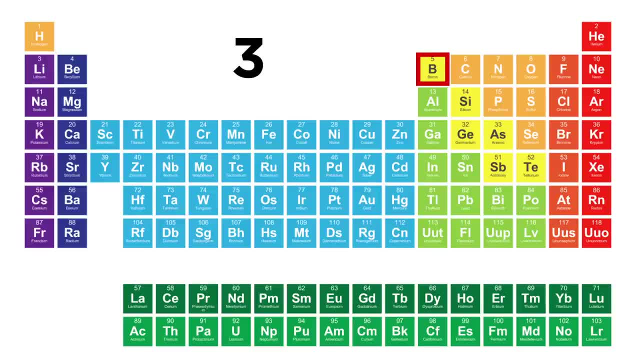 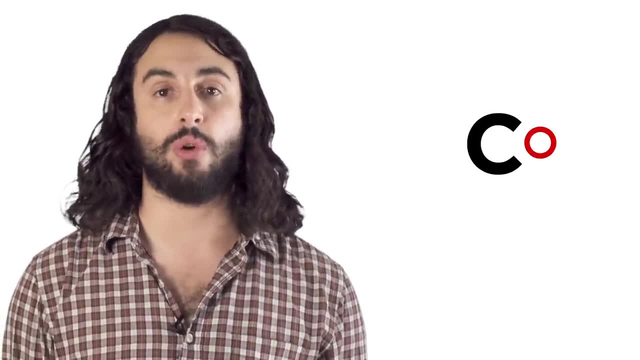 shell, which you can also tell by counting over from the left. for carbon and other small atoms, we assume that there are four coordination sites that can accommodate electrons or bonds, because this is how carbon can fill its octet or its outermost shell when we draw the valence. 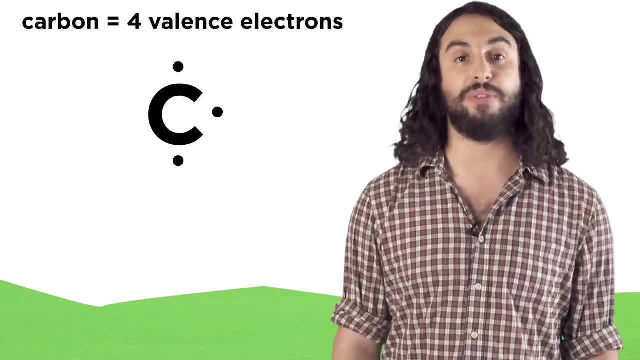 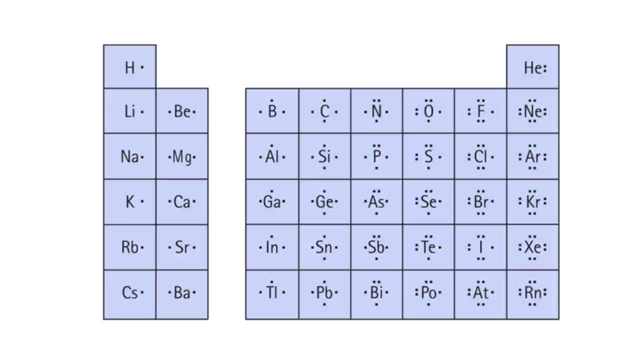 electrons. we put one in each coordination site first before pairing them up. so carbon will look like this, not like this. elements in the same group will have similar looking Lewis dot symbols because they have the same number of valence electrons. now to draw a. 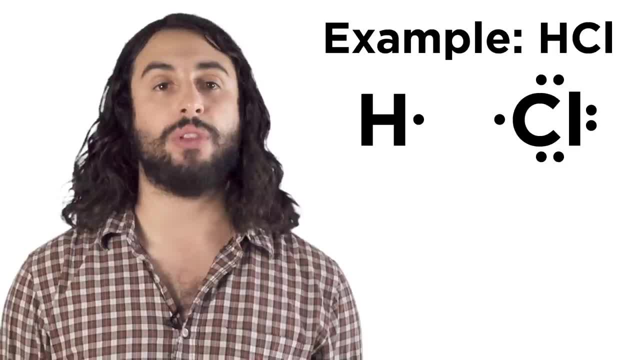 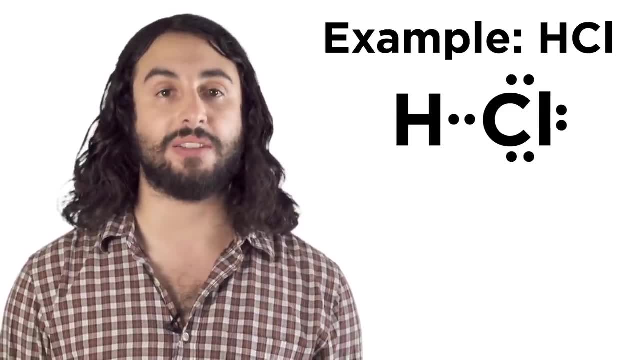 Lewis dot structure for a molecule. just draw each atom with all of its valence electrons. unpaired electrons from two different atoms can come together to make covalent bonds. when that happens, instead of two dots we make a line. this is a covalent bond which. 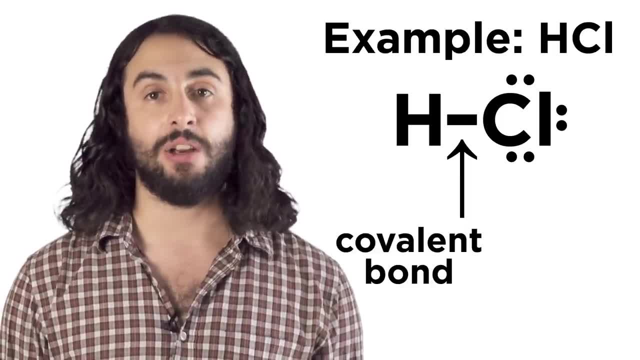 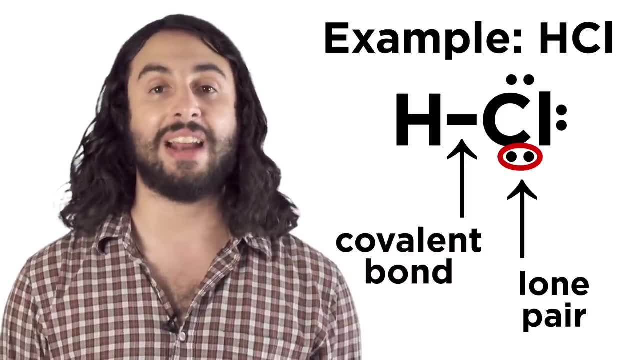 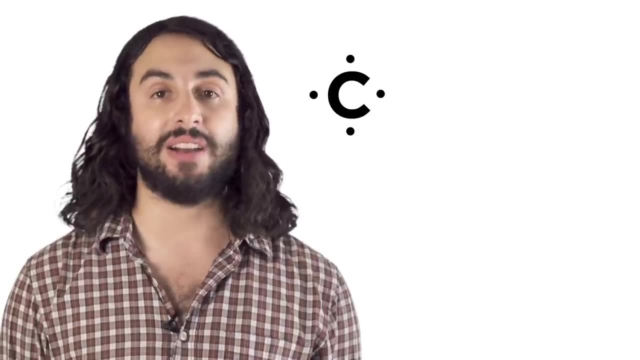 always contains two electrons. for our purposes here we can assume that electrons need to be paired. so a good Lewis dot structure will have all the electrons either inside covalent bonds or in lone pairs. the number of valence electrons an atom has dictates how many bonds it tends to form. 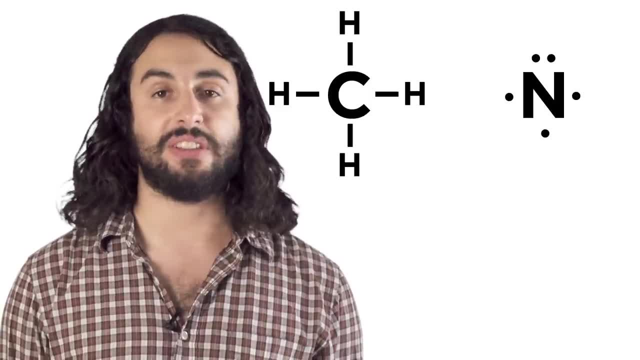 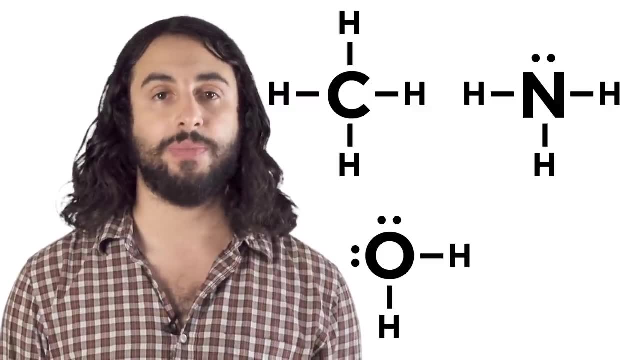 carbon likes to make four bonds. nitrogen, with five valence electrons, likes to have three bonds and one lone pair, oxygen likes to have two bonds and two lone pairs, and fluorine likes to have one bond and three lone pairs. when two atoms have one covalent 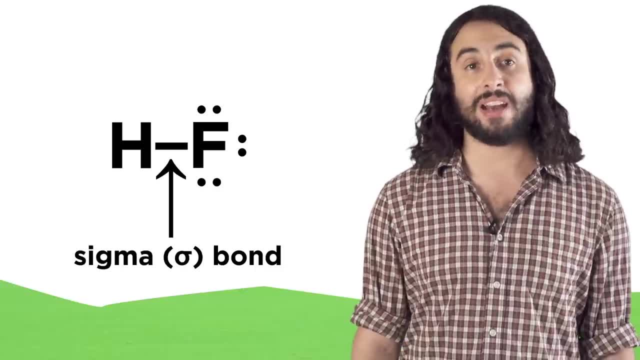 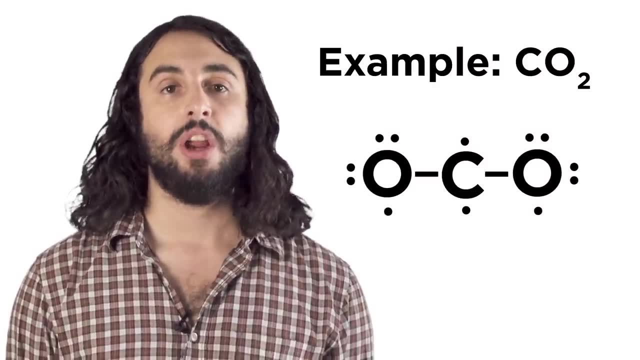 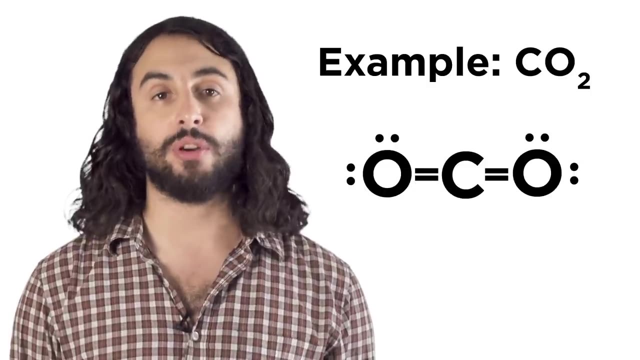 bond between them. we call that a sigma bond, but atoms can have double or even triple bonds. look at carbon dioxide. after we make a sigma bond between the atoms, there are still unpaired electrons. if adjacent atoms each have unpaired electrons, they can become another covalent.